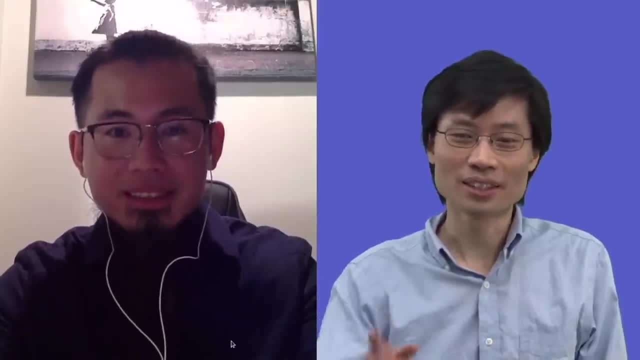 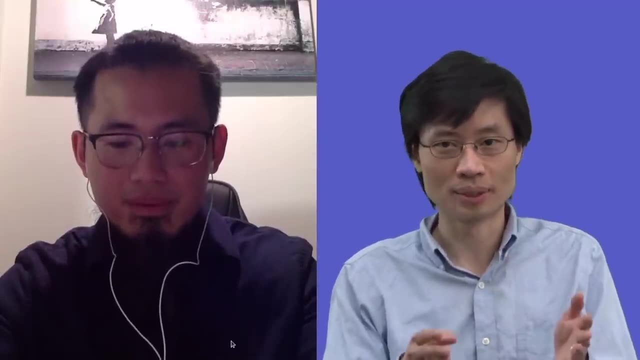 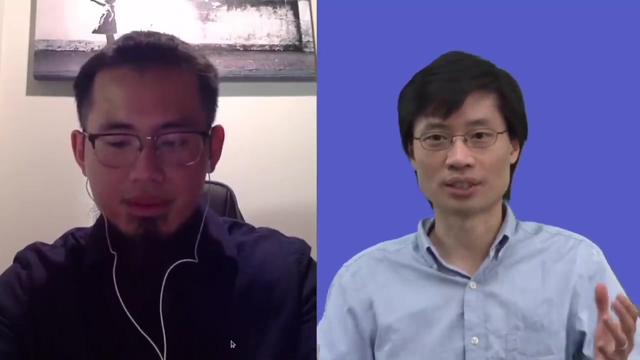 How do you prepare for math competitions? So here's a tip: If you want to prepare for math competitions, there's a different timeline of how close it is to the competition. If you are more than two months away from the competition, just focus on developing your skills in solving questions. 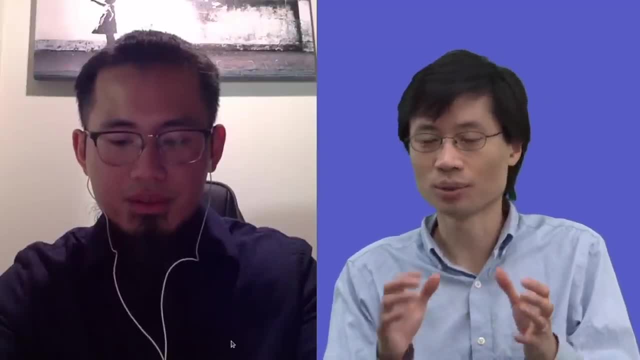 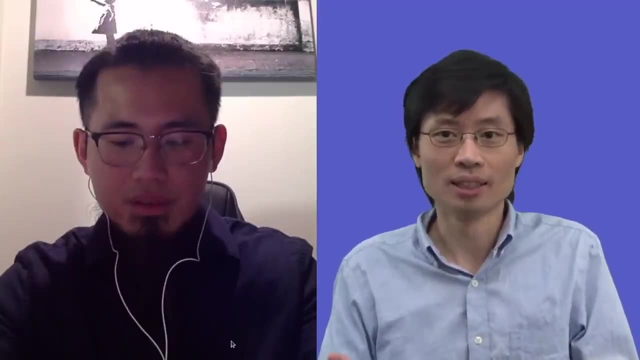 If you're within the last two months, start worrying about the actual speed and the time limits and everything in the contest. Here's why: Because a lot of people make a mistake where they prepare for a one-hour competition by always spending one hour and doing previous year's problems. 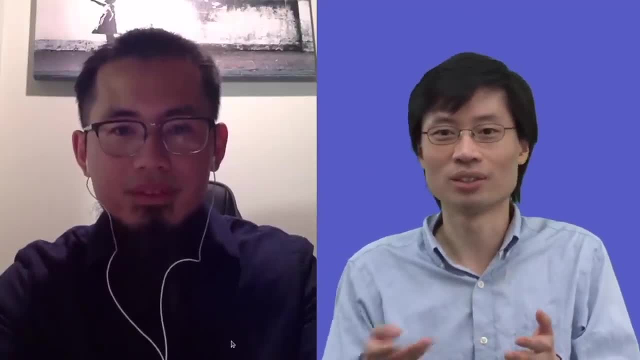 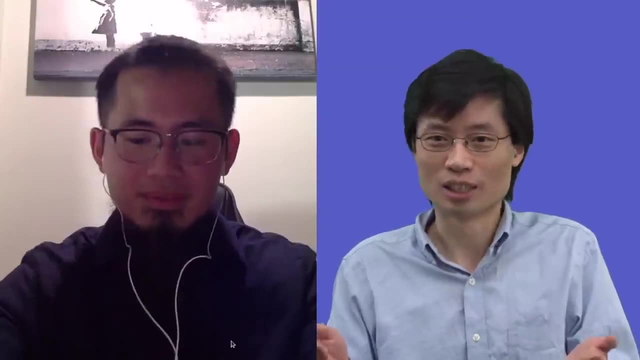 If you do that, you will only practice all the easy ones, which you already know how to do, And then you do some middle ones and you never get any time thinking about the hard ones because you ran out of time. But that's not making you better, It's just making you faster at the easy things. 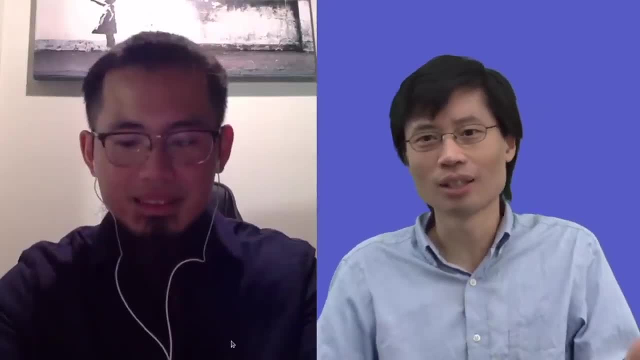 Much better is if you just use your time and say: I just go and do all the questions, I'll take a long time, Long time, Take a whole day, Even though it's a one-hour contest. But then you learn how to solve the hard things. 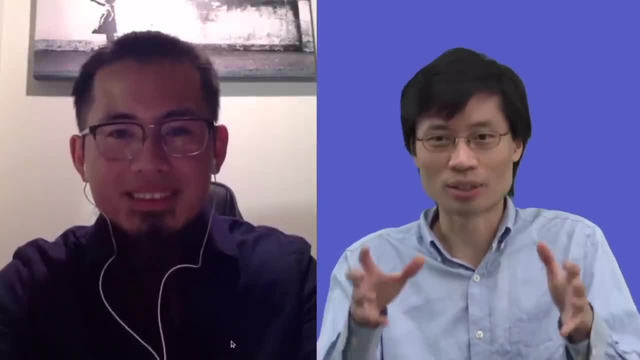 And then finally, finally, in the last two months, you go and say, okay, now I actually will go and learn how to do this in the time limit. 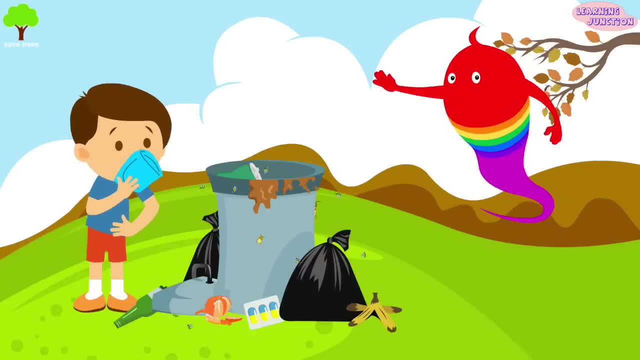 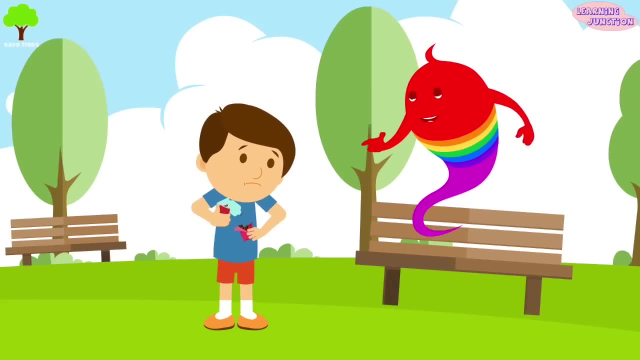 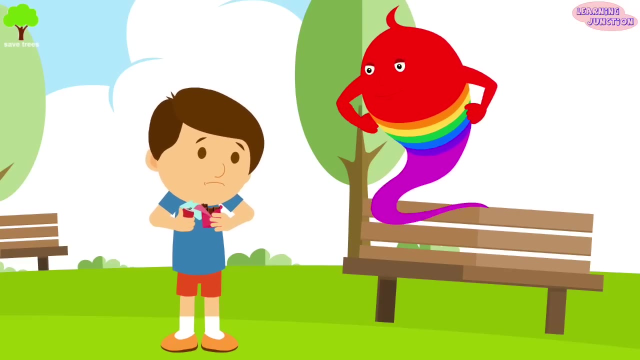 Hello friends, Today we'll learn about soil pollution. What do you do with your chocolate wrapper, water bottle or cola can? when you're finished with it, Do you throw it on the ground instead of into the bin? Yes, Ah, then you're contributing to soil pollution. 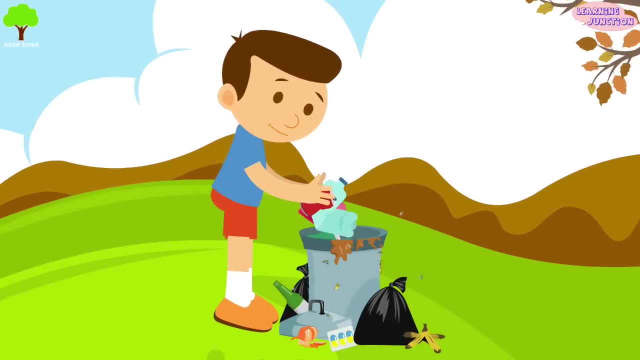 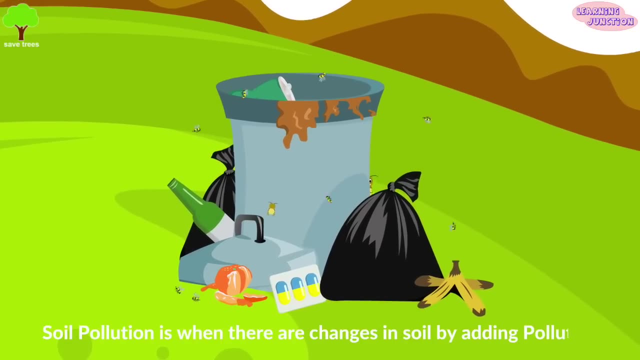 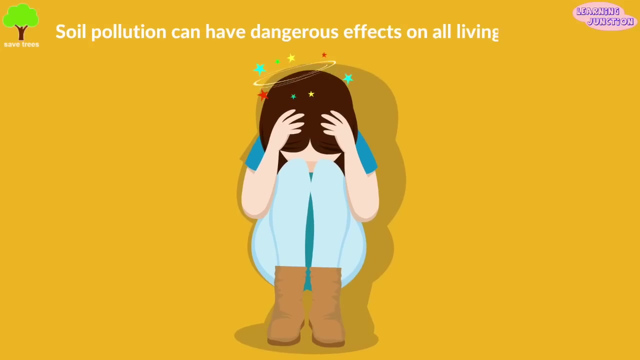 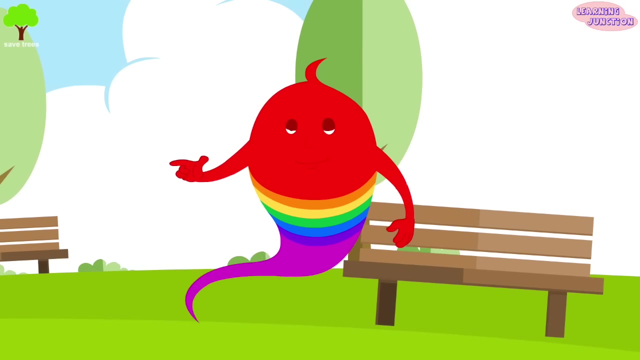 Soil pollution is when there are changes in soil caused by the adding unwanted and harmful materials or pollutants. Soil pollution can have dangerous effects on all living organisms, such as humans, animals and plants. Let's see some of the causes of soil pollution: Garbage throwing. littering systems and pollution. Soil pollution is when there are changes in soil caused by the adding unwanted and harmful materials or pollutants. Soil pollution can have dangerous effects on all living organisms, such as humans, animals and plants. Let's see some of the causes. dangerous effects on all living organisms, such as humans, animals and plants. Let's see some of the causes of soil pollution: Garbage throwing, littering systems and pollution. Soil pollution can have dangerous effects on all living organisms, such as humans, animals and plants. Let's see some of the